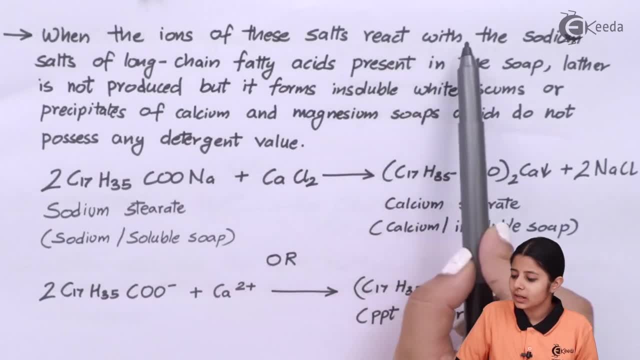 and we will see how it actually works When the ions of these salts react with the sodium, salt of long-chain fatty acid present in soap, lather is not produced, but it forms insoluble white scum or precipitates of calcium and magnesium soaps which do not possess any detergent. 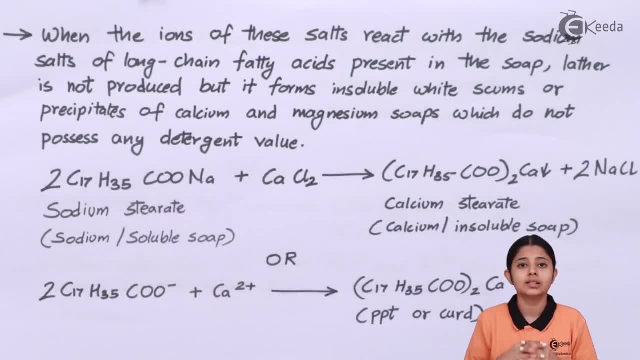 value. Let us see the examples of it now. what we are seeing in the examples of the reactions is: we are seeing hard water plus soap. So here I have twice or three times I have seen hard water plus soap. Now we see the reaction of hard water plus soap. So here I have: twice or three times I have seen hard. 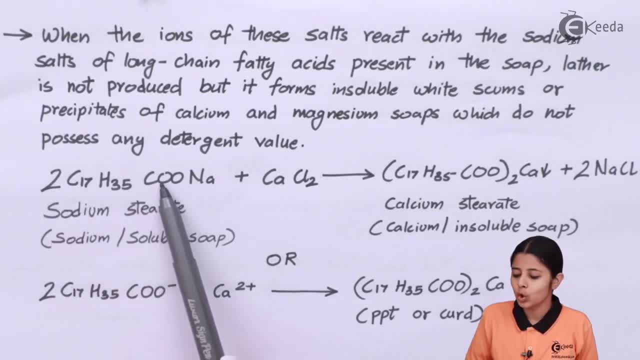 soap. what is soap? c17h35c double bond oona- this is the chemical formula of my soap, which reacts with cacl2, which is present in water. cacl2 present in water makes the water hard water. that means the water is hard water. now why? because calcium is dissolved in it, cacl2 is dissolved in it. this is 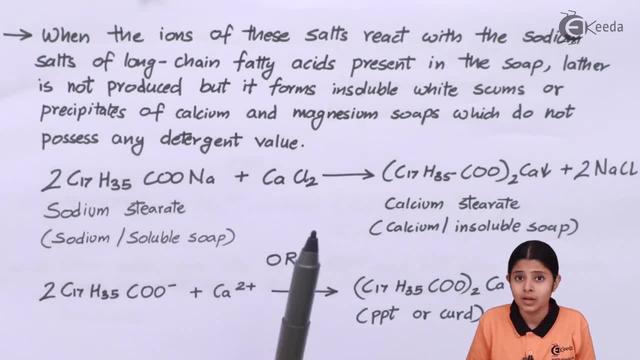 the dissolved form of water. this reaction is not between soap and water, but it's reaction between soap and hard water, and the hardness is due to cacl2. now, when this happens, this c17h35c double bond o, this part of it, which is twice, gets reacted with this ca, that is, calcium, forming a precipitate. 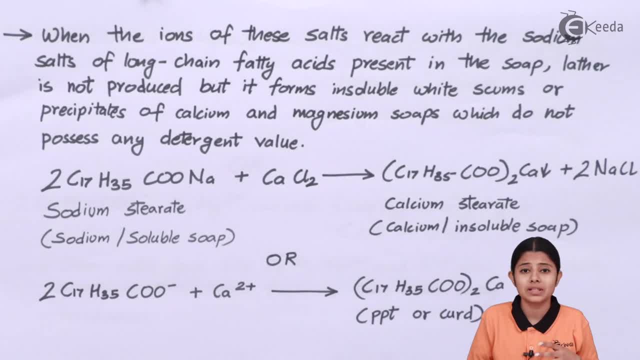 now over here we have to see that it's a precipitate and this precipitate is not lather. it's an insoluble precipitate which is a scum or a curd like substance. it is known as calcium stearate, that is, calcium insoluble soap plus twice of nacl. 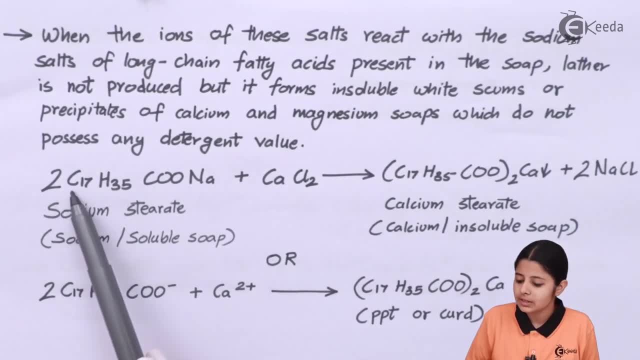 let us look at the balancing of this reaction. over here i have c17h35c double bond o o, which is twice, and this entire thing is there on the product side, c17h35c double bond o o, and over here it is twice as well. so this entire part of my soap is balanced over here. now let us see how. 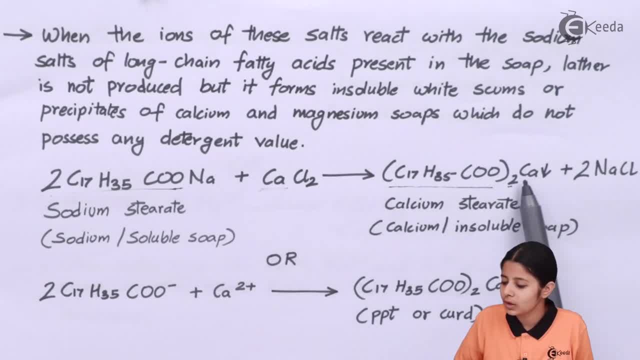 many calciums we have on this side, one calcium on the reactant side and one calcium on the product side. now we are still left with na from the reactant side. it is twice of na2na. so over here we will have 2na and plus cl2. so instead of cl2 we will have 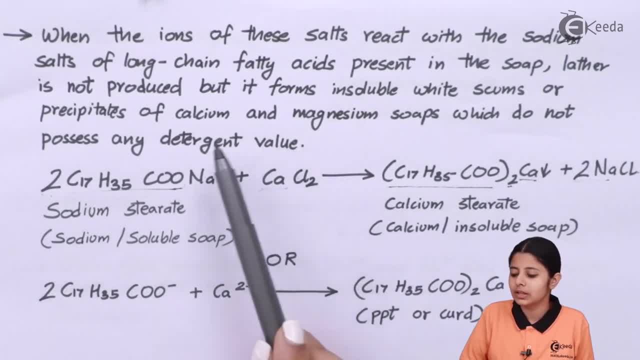 2cl, forming 2 nacl. so sodium stearate. when reacts with ca, cl2 forms calcium stearate plus twice nacl, and this is a balanced reaction. now, the same reaction we have shown over here, but in a form of ions. we are actually trying to say that na and cl is not playing a major. 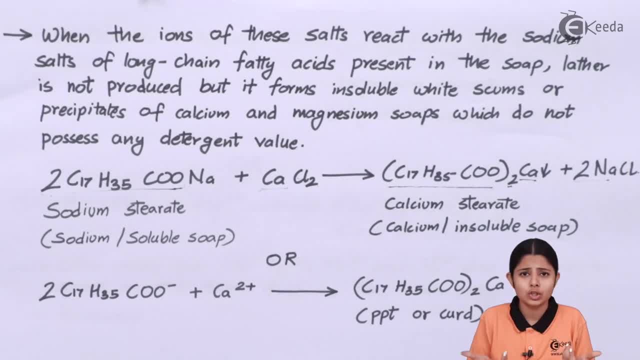 role because nacl is nothing but my sodium chloride. it's a very dissolved, we will salt water. what are the main ions? what are the main factors which lead to this reaction? are these? we have twice c17h35c double bond, o- o, which is has a minus sign, but this minus sign is into 2 because 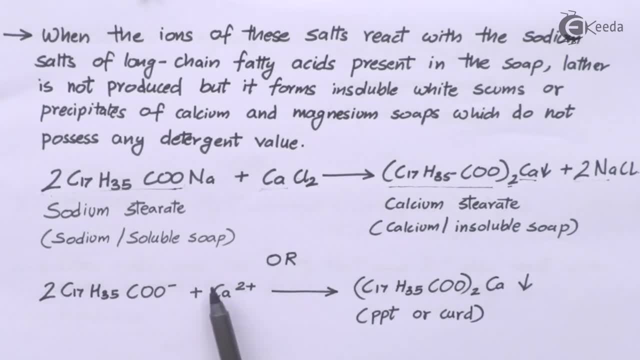 the entire reactant is twice plus ca2 plus. so over here i have two positive ions. i have a negative ion which is twice, and that's the reason why this will get substituted over here. this will get attached itself over here and it will form c17h35c double bond o- o, and this will get attached itself. 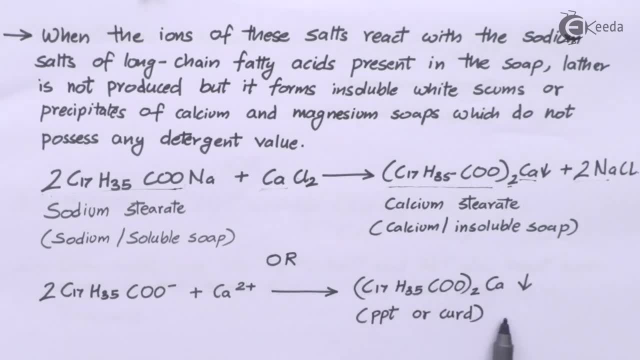 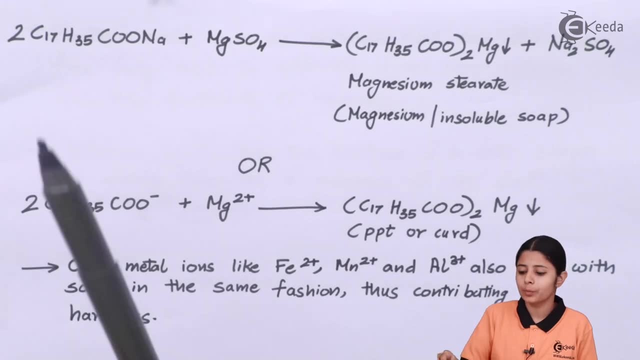 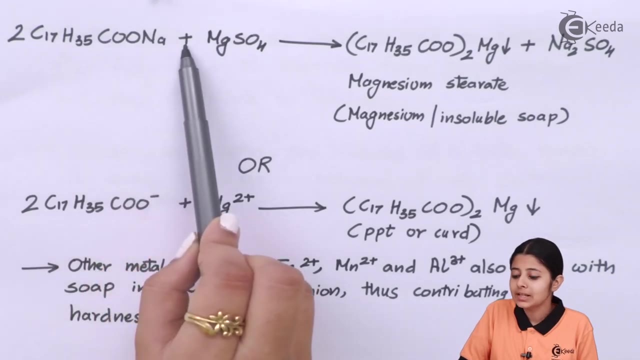 and this is nothing but my precipitate, also known as curd or scum. let us see the next reaction over here also, we are having soap. what is the chemical formula of it? c17h35c, double bond, o o, na plus mgso4. now this is hard water. hard water is because of the hardness of mgso4. 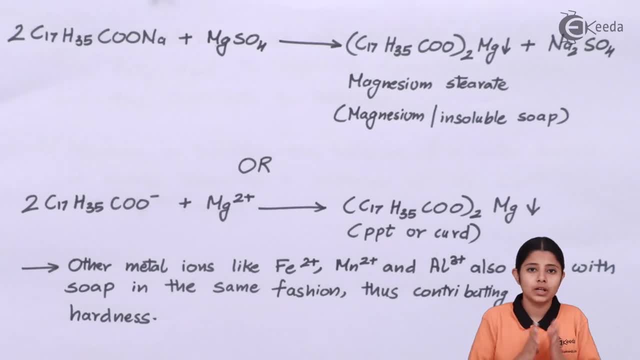 in the previous reaction it was because of the cacl2, but now we are using mgso4, so now soap will react with the mgso4. so let us see the entire reaction first and then we will see the ion form of the reaction. so we have soap plus mgso4, forming magnesium stearate plus na2so4 let. 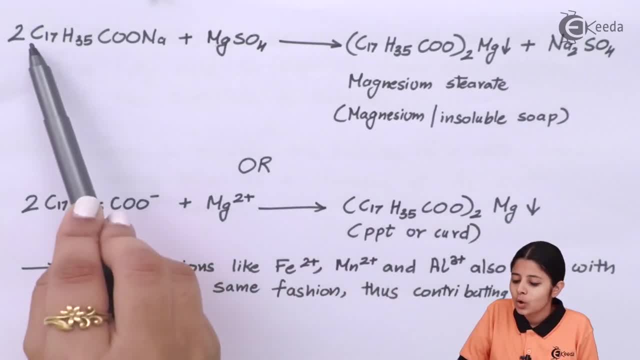 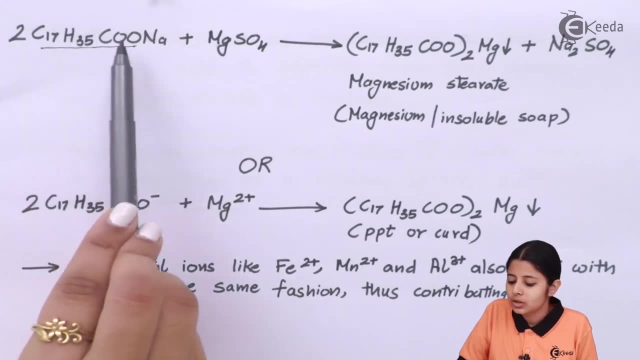 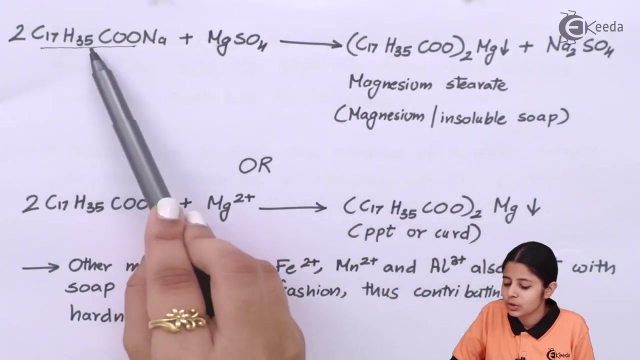 us see the balancing of this entire reaction and see how it is happening. over here i have c17h35c double bond o, which is twice. so this twice is over here c17h35c double bond o- twice. so this, which is on the reactant side, is same as it is on the product side, but over here i have two. 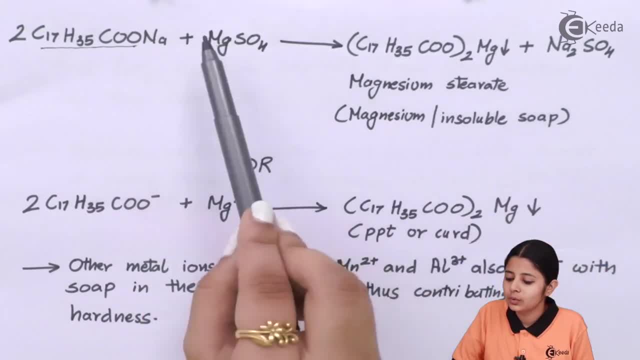 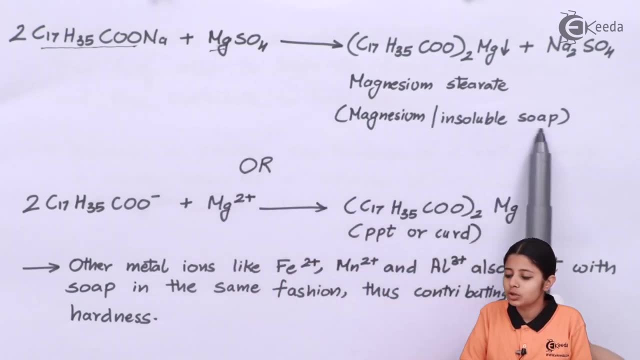 over here also, i have two. this gets reacted with mg. can you see? there is mg over here and it forms a precipitate. this precipitate is also insoluble soap, known as magnesium stearate. it is a curd or a precipitate form of it, and not lather of it. now, what is remaining on my reactant side is twice. 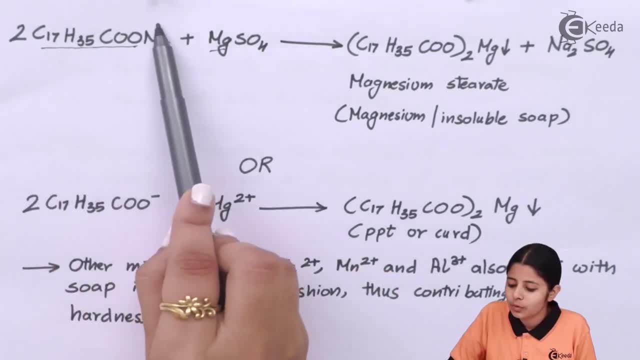 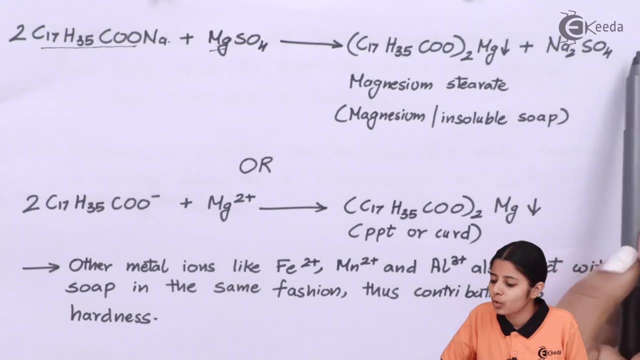 na and so4. the twice na comes from the reactant side, so this is twice na and so4. the twice na comes from the reactant, twice of na, plus over here i have so4, so this forms na2so4. now let us see only. 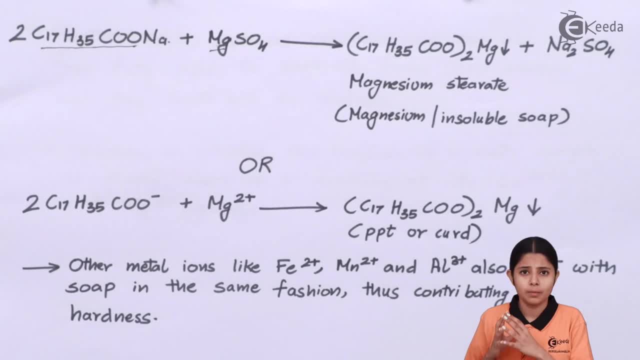 the ion form of the reaction, because of course na2so4 is just a byproduct. the main ions which take part in the reaction are the ions of the soap, obviously c17h35c, double bond o and minus over here, and it is twice, because over here we using it twice, plus mg2 plus. now why have i used? 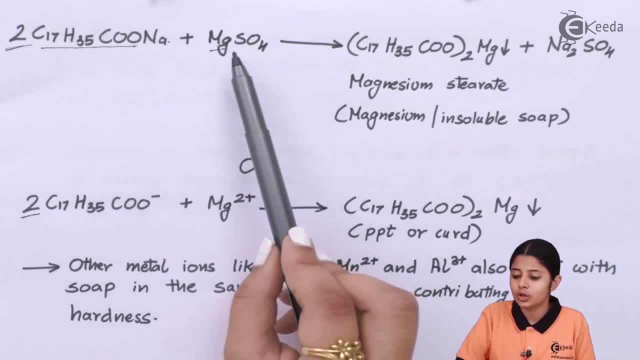 mg2 plus, because the valency of mg is 2 plus and so so4 is also 2 minus. so over here, mg2 plus, so4, 2 minus. the 2 plus and 2 minus used to cancel itself and mgso4 used to be a neutral, very neutral. in the same way, over here. 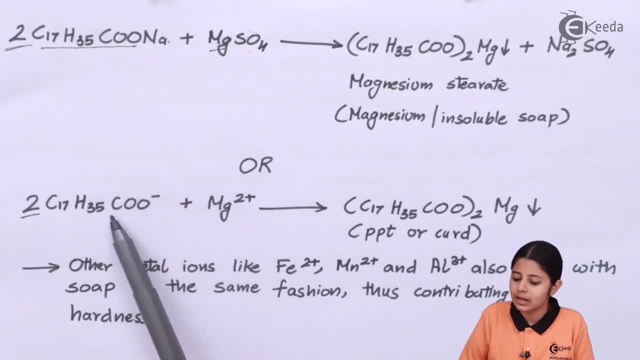 i have mg2 plus. this 2 plus will go and combine itself with c17h35c double bond o. so this on the reactant side comes here on the product side, forming c17h35c double bond o twice. why do i have mg2 plus, which combines with it and forms a precipitate or curd other metals like fe2 plus? 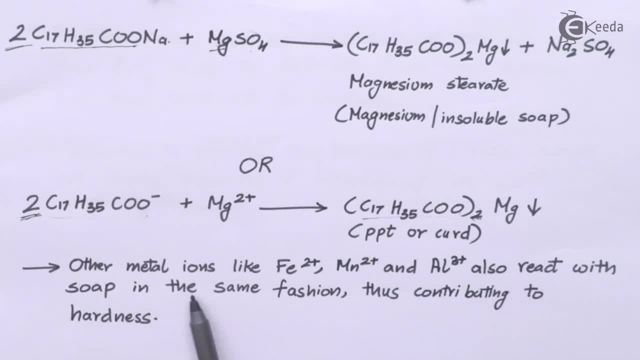 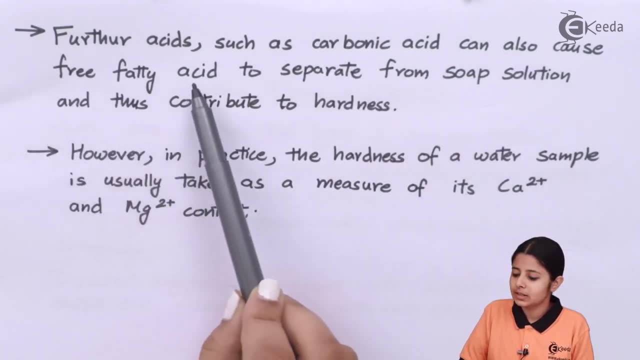 mn2 plus and al3 plus also react with soap in the same fashion, thus contributing to hardness. further acids such as carbonic acid can also cause free fatty acid to separate from soap solution and thus contribute to hardness. so it is not necessary that we'll have only calcium or magnesium salts. 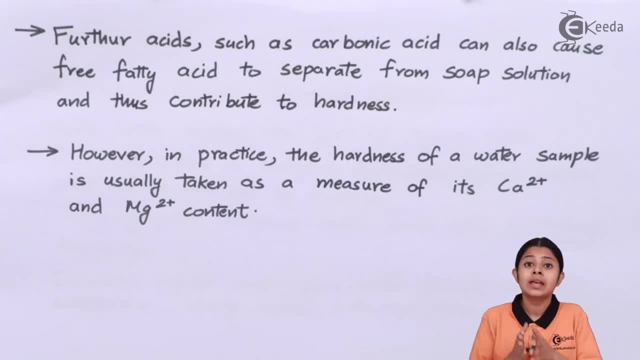 we can have iron salts, manganese salts, aluminium salts, and apart from all of these, we can also have carbonic acids, which are present in water. water is not distinguished as hardwater only because of carbonates or bicarbonates of calcium, magnesium, aluminium or iron. it can be also distinguished. 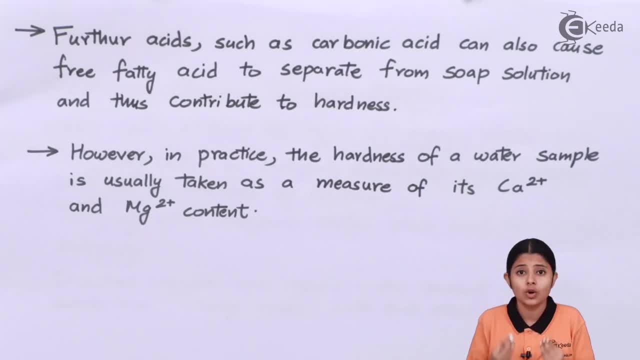 as hardwater because of some dissolved gases present in it. even dissolved co2 present in water can lead to hardness of water. so it is very important for us to know that it is not only certain salts but many other factors which lead to hardness of water. however, in practice, the 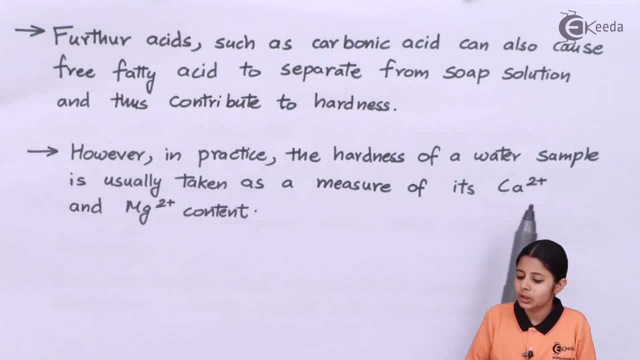 hardness of water sample is usually taken in a very severe situation and will not be able to taken as a measure of Ca2 plus or Mg2 plus content, because calcium and magnesium are two most important factors, are two most important elements and most commonly found elements in hard water.